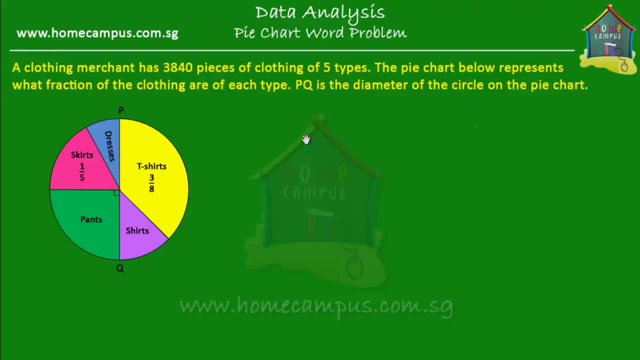 PQ is the diameter of the circle on the pie chart. Okay now, PQ is the diameter of the circle, And what does the diameter do? Well, a diameter divides the circle into two halves. So in the case of this pie chart, it divides the pie into two halves. 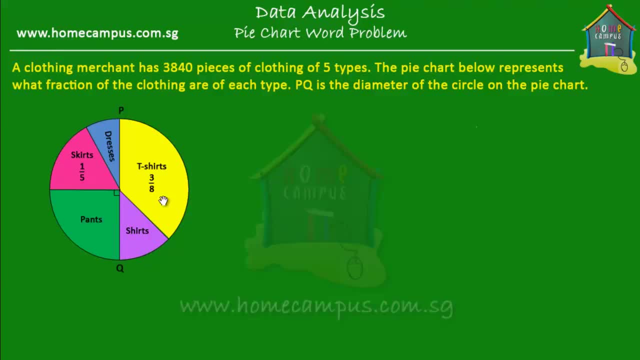 So the t-shirts and the shirts. together they constitute half the clothing, And the dresses, skirts and pants constitute the other half of the total number of pieces of clothing. Okay, now, what can we tell about this slice of the pie over here, the green one that represents the pants? 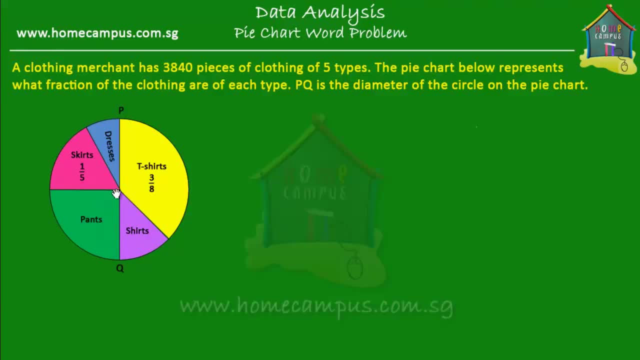 Well, what we can tell is, looking at this slice and this right angle over here, we can tell that this is a quarter of the whole pie chart. So the pants are one fourth of all the pieces of clothing. All right, now let's look at our questions one by one. 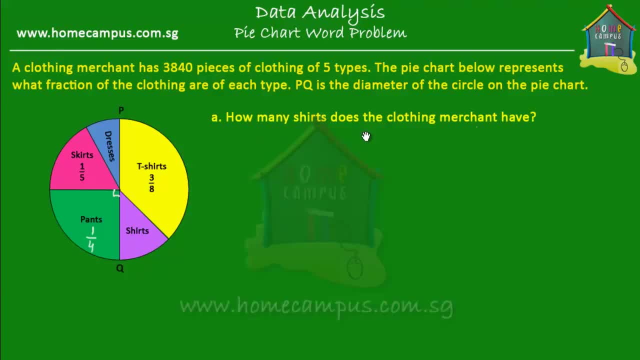 Let's see what the first question is. It says: how many shirts does the clothing merchant have? Okay, the shirts are here. Now we don't know what fraction of the clothing is shirts, but we can find that out easily. How Well we know that? the t-shirts and the shirts together, they are half. 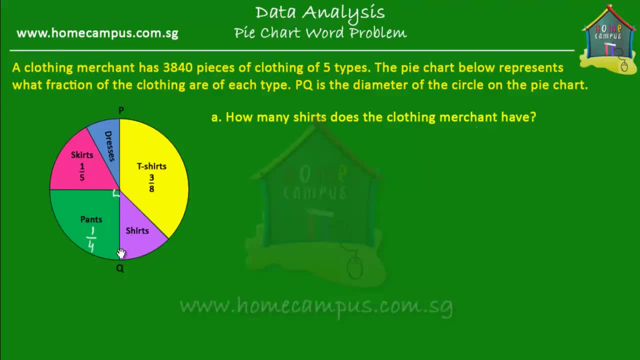 of all the pieces of clothing. Why? Because PQ is the diameter, and that diameter divides the pie into two halves. okay, So the t-shirts and the shirts together are one half. So how do we find out what fraction of the clothing is shirts? 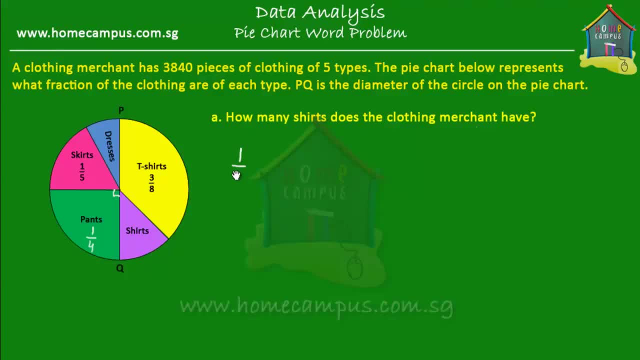 Well, you simply subtract the fraction that is t-shirts from half, and then you will get the fraction that is shirts. okay, It's quite easy. Well, one half can be written as 0.8,. then you subtract 3.8 from 8, and what you will get is 1.8, right. 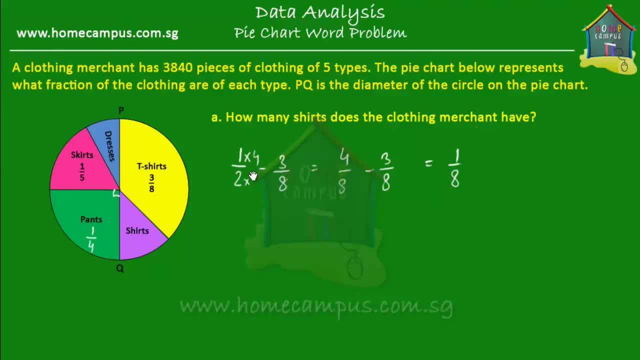 One half. how do you get 4.8?? Well, you multiply that by 4, and this also by 4, so you get a common denominator: 8 here and 8 here, and then you subtract. We know that bit about fractions. 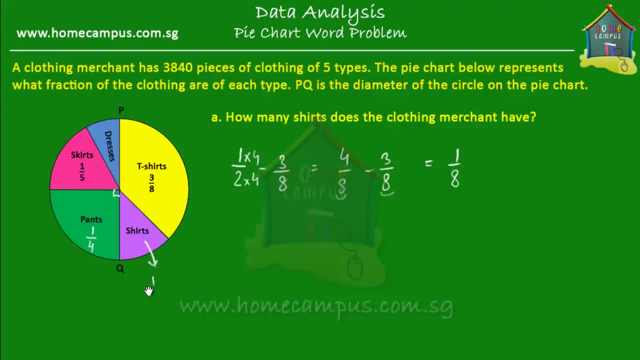 All right. so 1.8 of all the clothing is shirts. and if there were 3,840 pieces of clothing altogether, then what is the number of shirts? Well, 1.8 of 3,840 is shirts. So that means 1.8 of 3,840 is shirts. and let's see, let's just 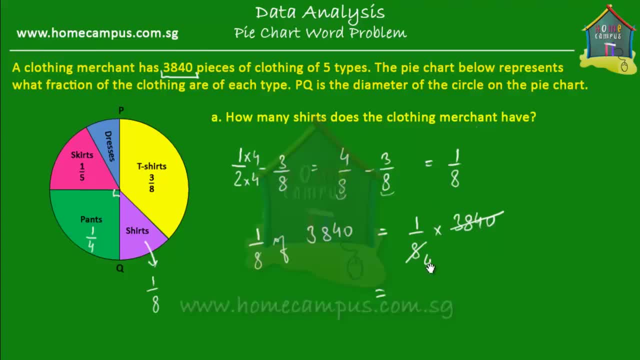 simplify this. How do we do that? Well, divide this by 2, you get 4.. Divide this by 2, you get 1, 9,, 2, 0. Divide that again by 2, you get 2 here and you get 19. divided by 2 is 9.. 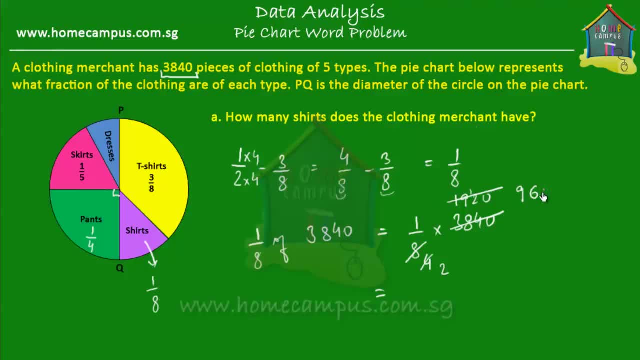 You have one remainder which you put here, and this is 960.. This can again be divided by 2.. We do that. This gives us 1, and this gives us 4.. You have a remainder of 1,, 8, and 0.. 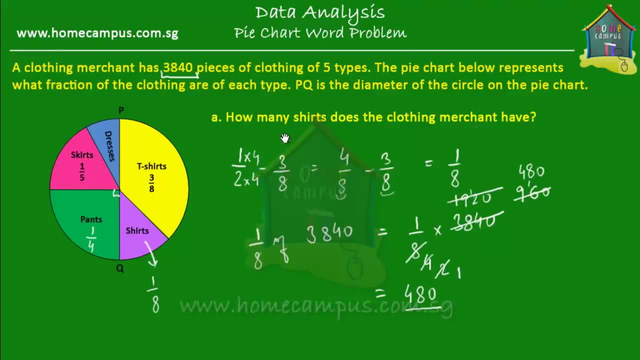 So there were 48, eight t-shirts. Okay, That's the answer to the first question. Let's move on to the next question. All right, The next question is: what fraction of the clothing are dresses? All right, Before I forget. 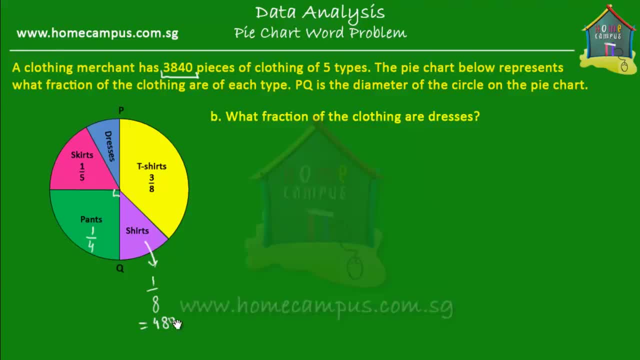 me write that number here. the shirts are equal to 418, number. all, right, now the fraction of clothing that are dresses. let's see, the dresses are here. okay, let's find out what this fraction is equal to. well, we know that again, the pq, the diameter, divides the pi into two halves. so the dresses. 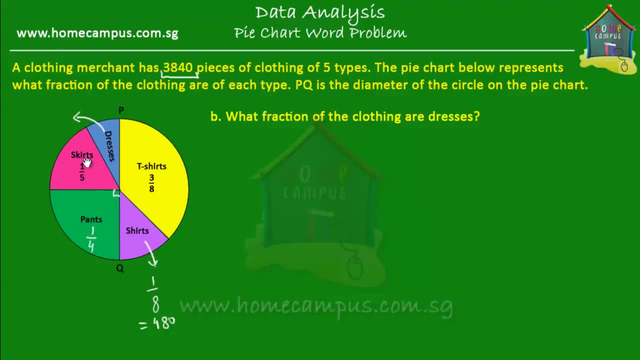 plus the skirts, plus the pants, is one half of the pi right now. how do we find out what fraction of the clothing addresses? so, again, simply, just like before: half minus the fraction that is skirts, is one fifth minus the fraction that is pants, which is a quarter. right, but we know this is a quarter. 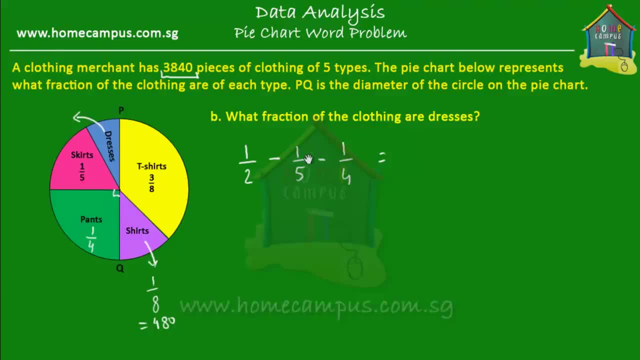 because of this right angle mark, right, all right. so one half minus one fifth minus one fourth, let's find a common denominator. the common denominator is 20, right? so times 10 times 4 and times 5 times 10 here is well, times 4 here as well, in this times 5. so 10 over 20 minus 4 over 20 minus 5 over 20. 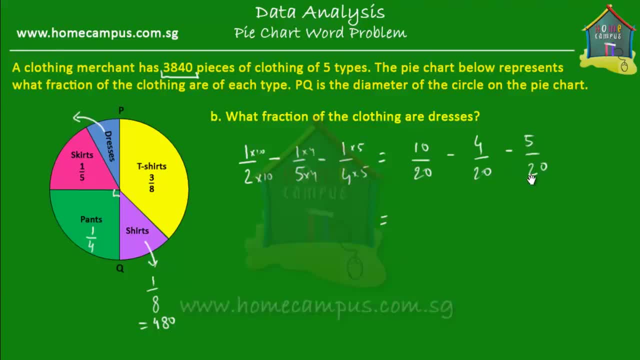 all right now. if you don't know how to find common denominators and all that stuff, then please go watch the videos that I did on now fractions and you will know how to get common denominator. all right now. 10 minus 4 minus 5, what is that equal to? that's equal to 1. 10 minus 4, 6, 6 minus 5 is. 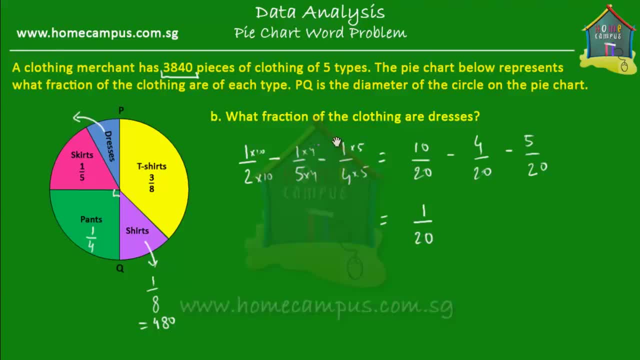 1. So this is 1 over 20.. The fraction of the clothing that are dresses is 1 out of 20.. So that means that if this pie was taken and cut into 20 small pieces, then one of those pieces would be the fraction that represents the dresses. All right, that's it. It's quite easy, Let's move. 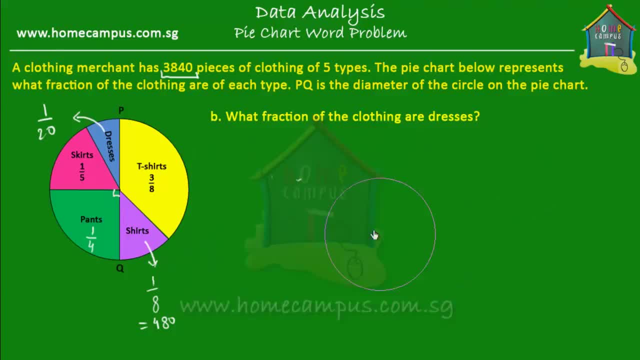 on to the third question, And the question is: how many dresses are there? Well, this is quite simple. We know that 1, 20th of all the clothing is dresses. Then, to find out the number, we simply do 1, 20th of 3,840, because there are 3,840 pieces altogether. So the 0 and the 0 cancel out. 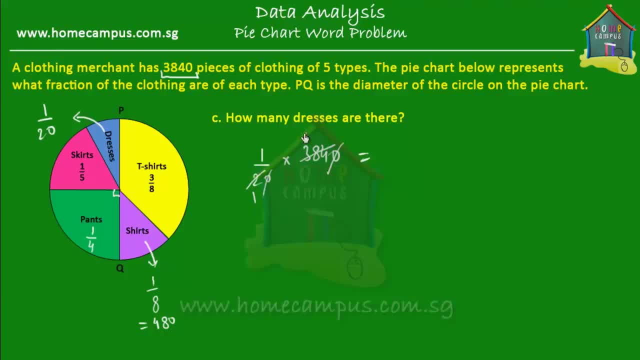 Then you divide this by 2, you get 1.. You divide this by 2, you get what Let's see: 1. You have a remainder of 1.. This is 9.. And this is again 2. So it's 192.. So 192,. 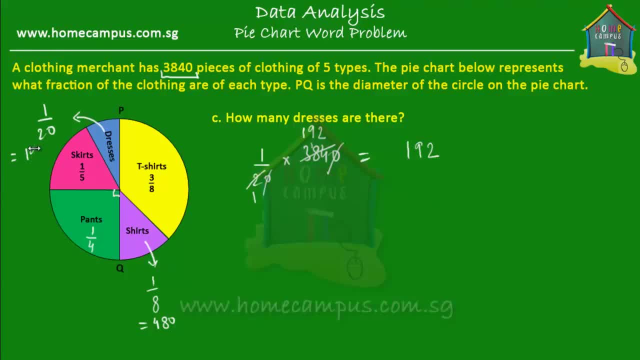 pieces of clothing were dresses. Quite simple, right? Let's see what the next question is. Well, the next question is: are there more dresses or skirts? How many more? Well, let's see, The skirts are here, The dresses are here. It's quite obvious that the slice that represents the skirts 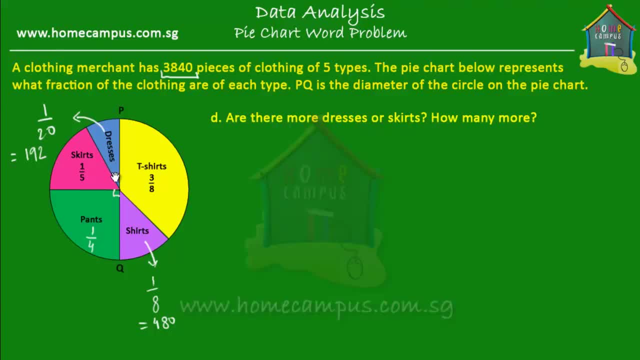 is bigger than the slice that represents the dresses. Now, you have to keep in mind that a pie chart is always drawn to scale, which means that if there are more skirts than dresses, then the slice that represents the skirts has to be bigger than the slice that represents the 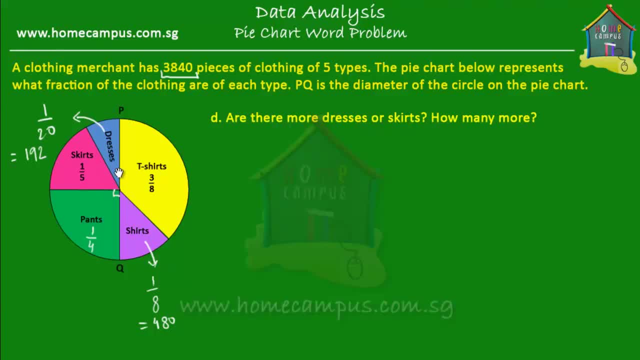 dresses. okay, So it's always drawn to scale. So from this pie chart we can tell quite easily that the skirts are definitely more in number than the dresses. And also, you know, if you look at the fractions, the fraction for the skirts is 1, 5th right, This one over here, And the fraction that 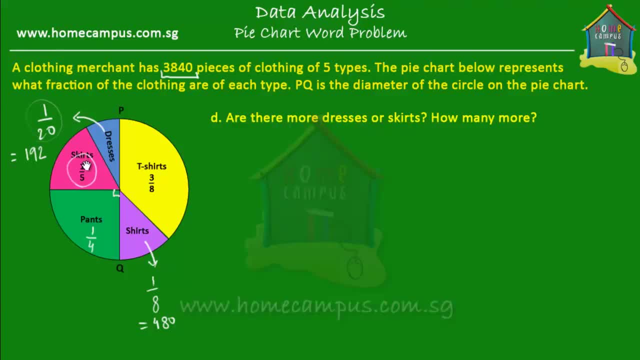 represents the dresses is 1: 20th And we know that 1: 5th is bigger than 1: 20th, So obviously there are more skirts than dresses. Now that we know that there are more skirts than dresses, we have to find out how many more okay? 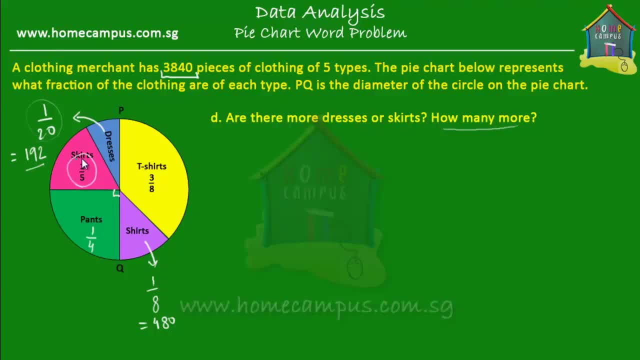 We know that there are 192 dresses, but how many skirts are there? Well, 1 5th of all the clothing is skirts. So 1 5th of 3,840 is skirts. What is that equal to? Let's simplify this: This is 7. 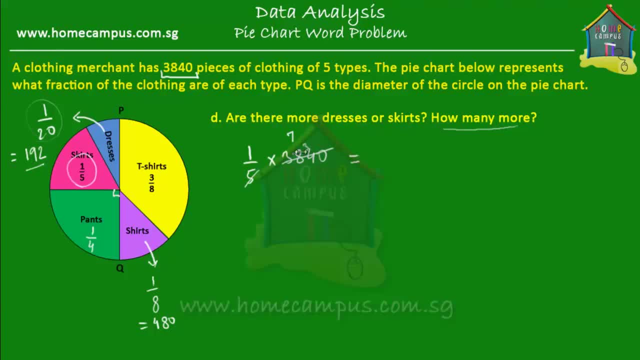 times 5 is 35.. You have a remainder of 3.. 5 times 6 is 30.. You have a remainder of 4, and 5 times 8 is 40,. okay, with no remainders. So 768 pieces of clothing are skirts. 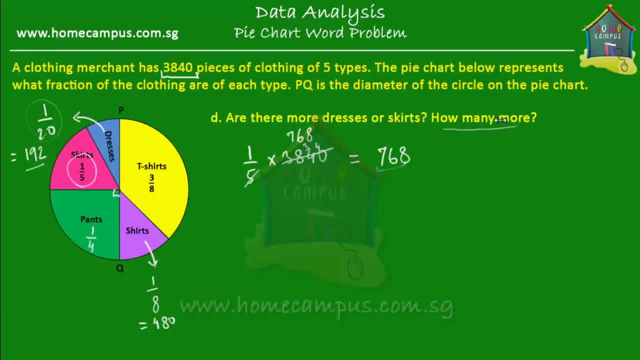 so there are 768 skirts. Now we have to find out how many more. so we simply do 768 minus 192, because there are 768 skirts and 192 dresses, and that will give you, let's see, 8 minus 2 is 6,. 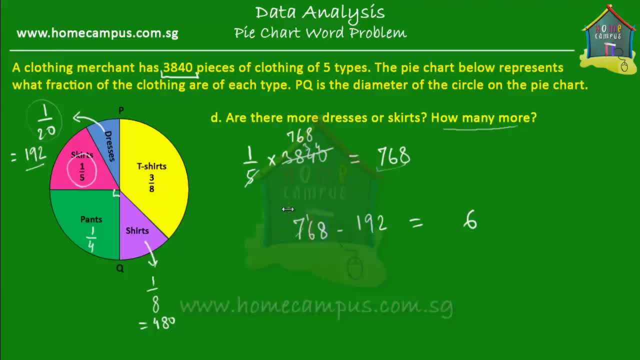 16 minus 9 is 7,, 6 minus 1 is 5, so there are 576 more skirts than dresses. That's the answer to this question. how many more? All right, quite easy, let's see what the next question is. 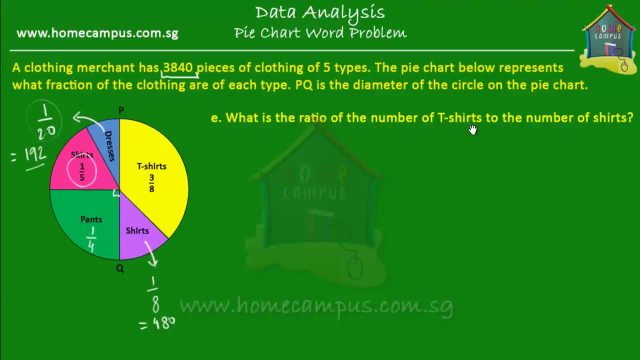 All right. so the question is: what is the ratio of the number of t-shirts to the number of shirts? Well, we know that the number of shirts is 480, but do we know what the number of t-shirts is? Well, we don't know yet, but let's find out. Three-eighth of all the clothing is t-shirts. 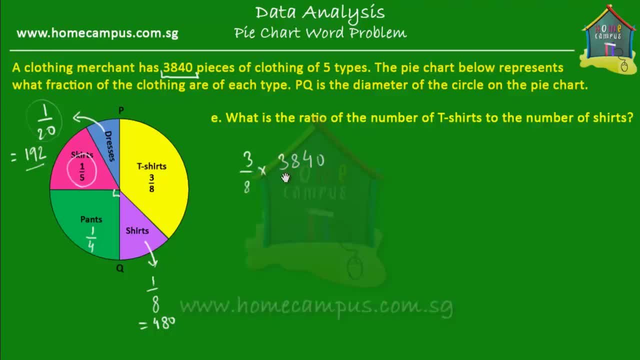 so 3,840 is all the clothing. Three-eighth of that is t-shirts. so let's find out what that is equal to. Well, how about I use a calculator to be quick? So 3,840 times 3,, okay, whatever that is divided by 8 is 1,440.. So 1,440, that's the number of t-shirts, okay. 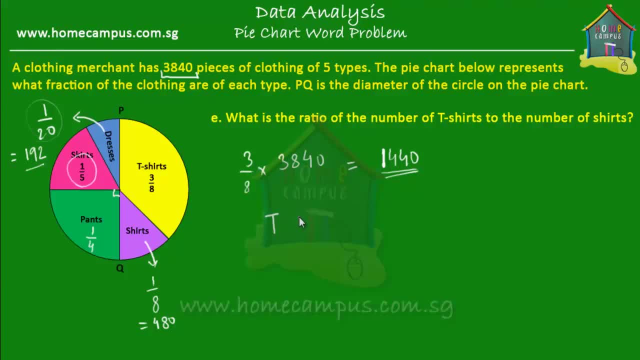 Now we have to find out the ratio of the number of t-shirts to the number of shirts. So 1,440 is the total number of t-shirts and 480 is the total number of shirts. How do we simplify this? Quite easy. 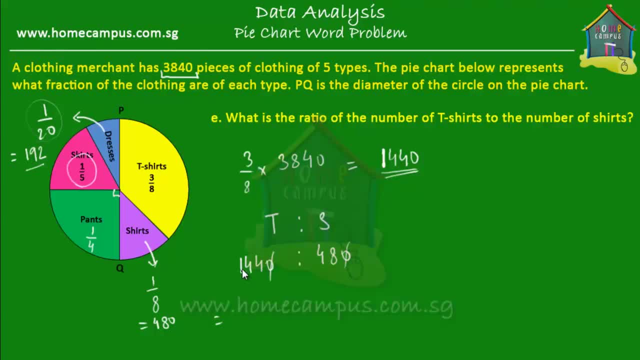 Well, 0 and the 0 cancel out 144,. we know that's divisible by 12, because 12 times 12 is 144, and we divide this also by 12,, we get 4.. So the new ratio is 12 to 4, which can again be simplified. 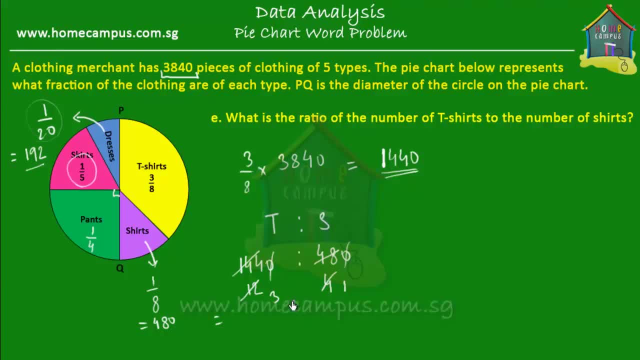 Divide this by 4, you get 3.. Divide this by 4, you get 1.. So the ratio of the number of t-shirts to the number of shirts is 3 to 1.. But there's another way of finding that out, You know. 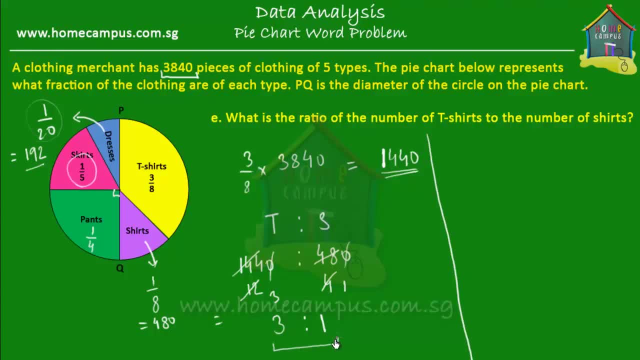 if you don't really go and find out what the total number is, you can use the fractions and you can come to the same answer. You know how Well. 3 eighths of all the clothing is t-shirts and 1 eighth of all the clothing is 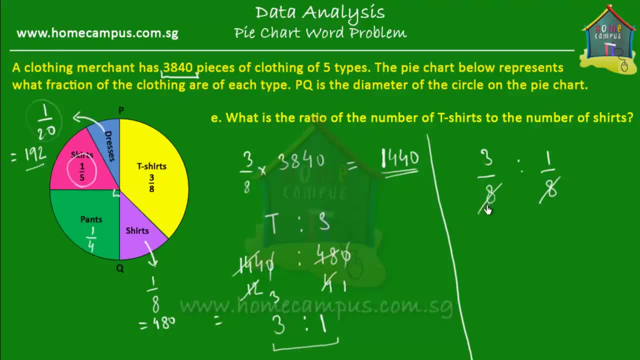 shirts. Now cancel this out. cancel this out because they're both 8.. What you're left with is 3 to 1, and that's the same as this answer over here that we got to using the number of t-shirts. 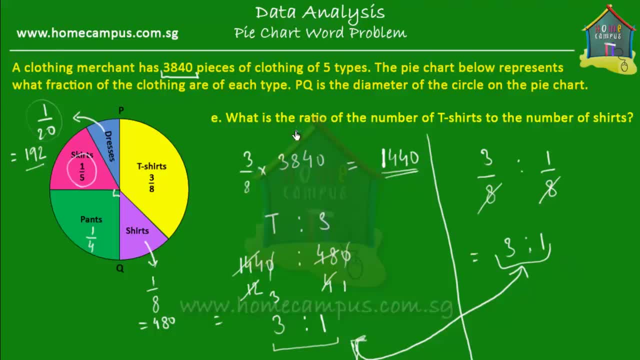 and the number of shirts. So if it's just the ratio that you have to find out, then it doesn't matter whether you use the actual numbers or the fractions. You should get the same answer, because all you care about is the relation between the two right Between the number of t-shirts and the number of shirts. 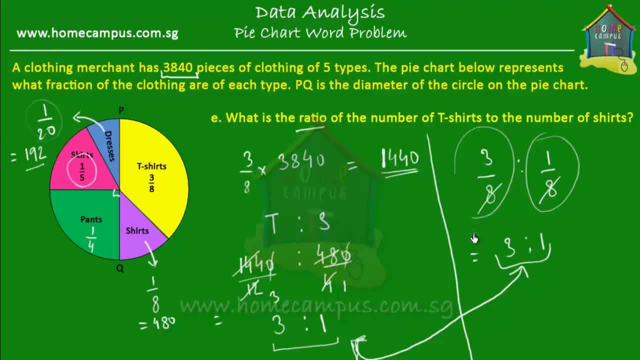 So you can use either fractions, or you can also use percentage, if that's given to you, or you can use the number, and you will still get the same answer, In this case 3 to 1.. All right, Okay, next let's see. 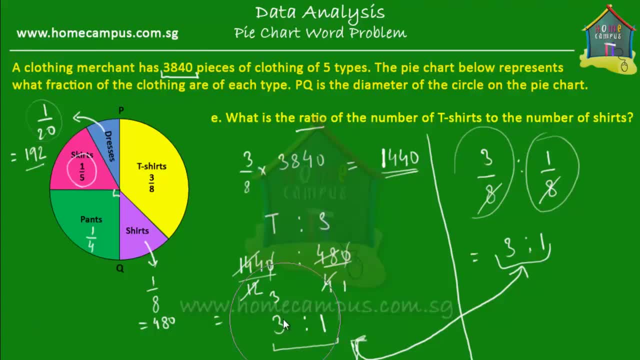 I think there's one more question. Let me make some room here and find out what that is and then solve it. Okay, All right, How many percent of the clothing are pants and skirt? We have the skirts here. The fraction is one-fifth, the pants is one-fourth. What we have to find out is the. 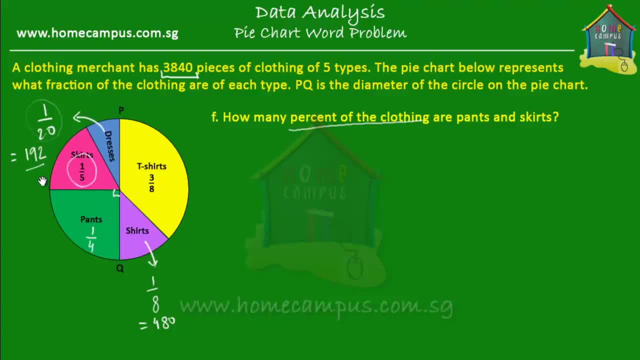 percent of the clothing that are pants and skirts. Okay, let's see what fraction of all the clothing is skirts and pants together. So pants is a quarter and skirts is a fifth. Now let's see. Let's find a common factor. 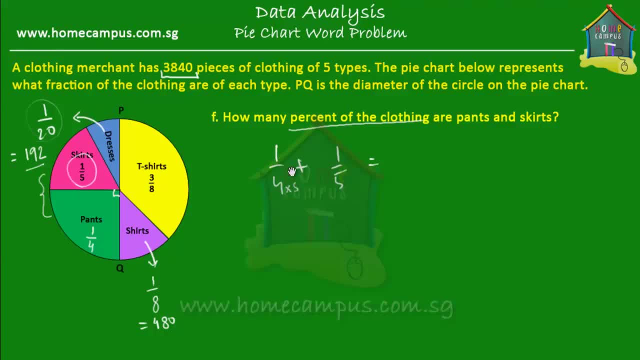 a common denominator. actually, This is times five, Five times five, This is times four times four. So the common denominator is 25 over 20 plus four over 20.. So, nine-twentieth, of all the clothing is either pants or skirts. Okay, So that's the fraction.